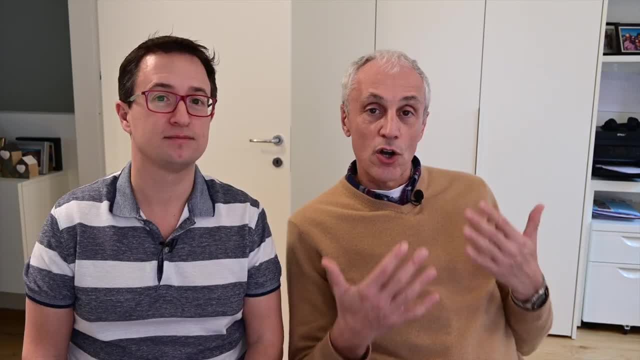 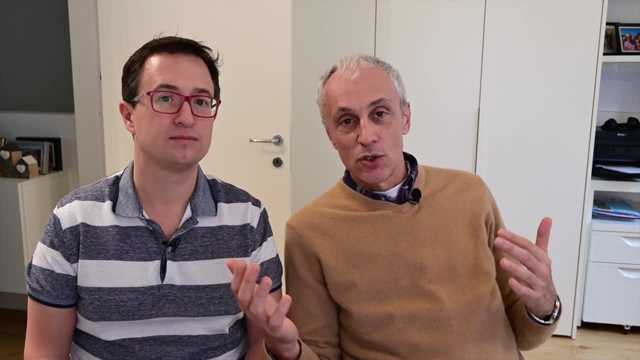 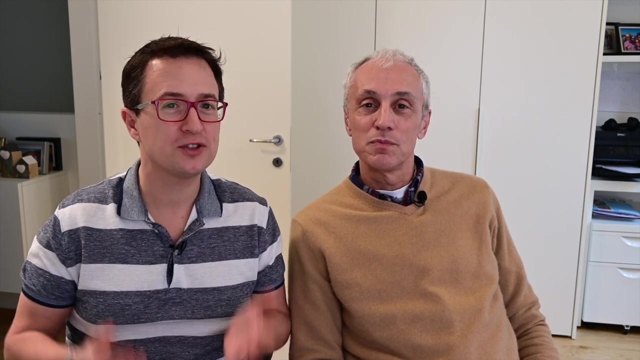 Istanbul, and then there's a combination of the two and generally longer cruise, 15 plus days, and they're called Mediterranean Medley or Mediterranean Explorer, and they can go from Barcelona to Athens or vice versa. they are fun. so you might be wondering which ports are the best to visit in the Mediterranean. 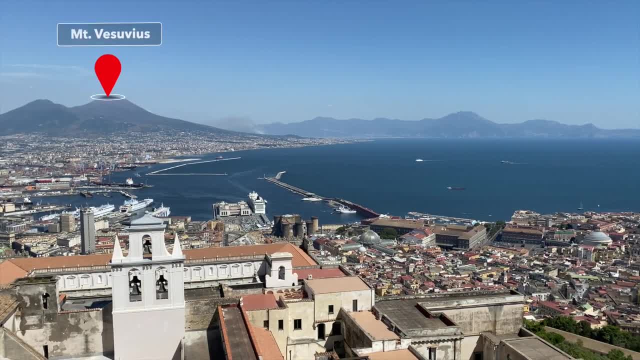 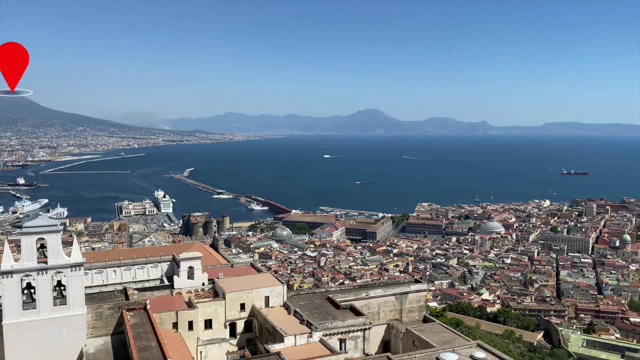 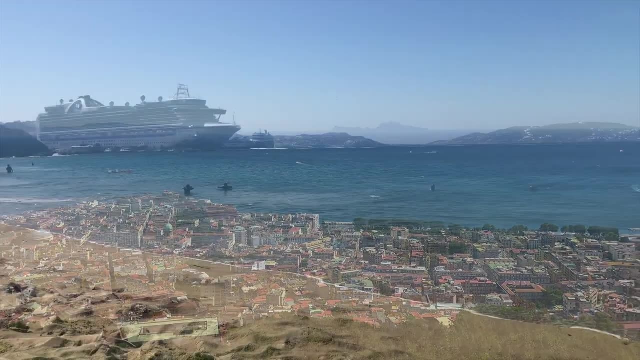 well, every port is pretty unique and it has, you know, lots of wonderful things to see. in general, the Western Mediterranean ports are more for people looking to visit cities and cultural and archaeological sites. Yeah well, the Eastern Mediterranean cruises are better for people looking to. 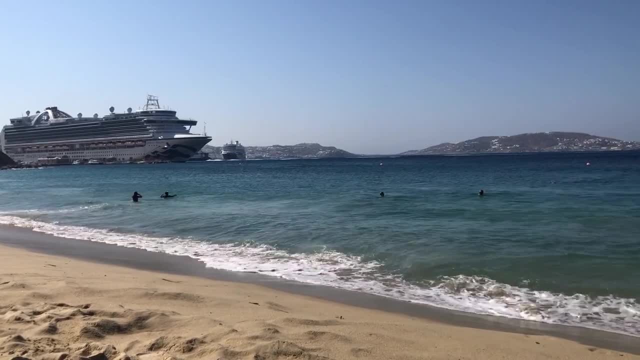 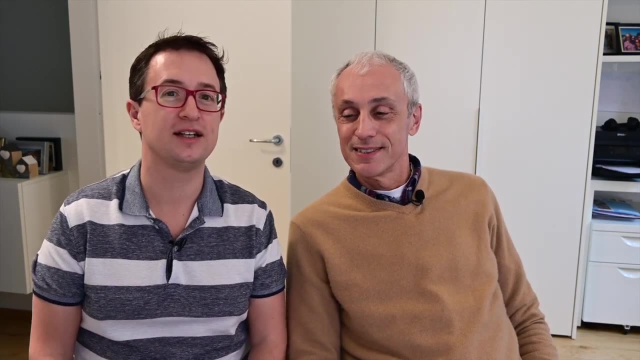 relax on the beach or swimming in the mud in the nice meet Greek islands. so these are the difference, the main difference, and now let's explore which one are our favorite port. Oh yeah, great idea. So let's start from the Western Mediterranean Ports in the Western Mediterranean that we like are Barcelona. 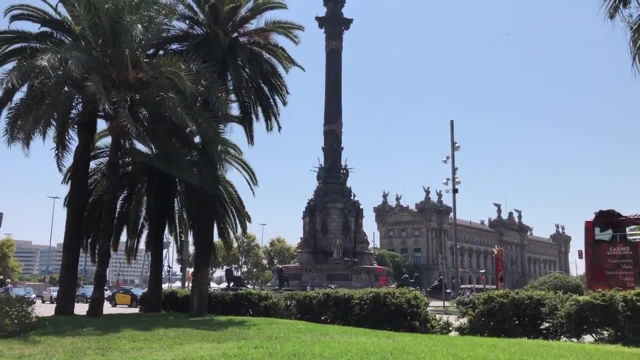 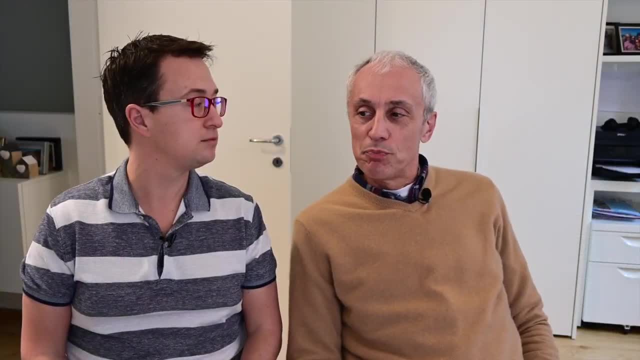 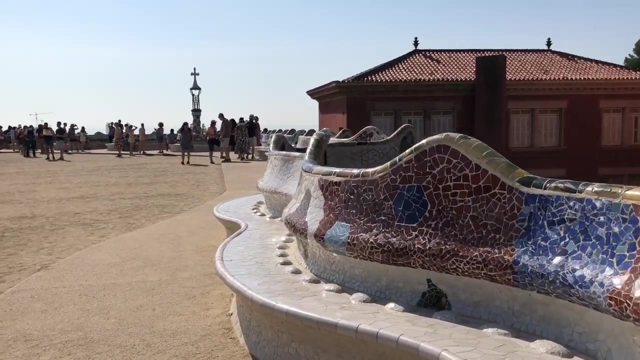 Barcelona is beautiful. Yeah, you don't need a car, you just go. Yeah, you don't need a car, You just walk from the port. Actually, we went J seguir yeti to park. go well, yes, park of well, park. well, it's a very famous park in barcelona, designed by gaudi. 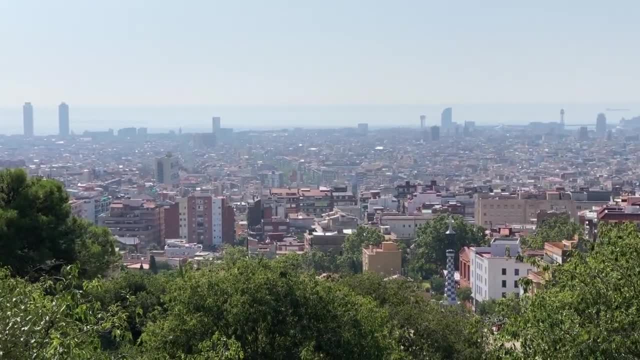 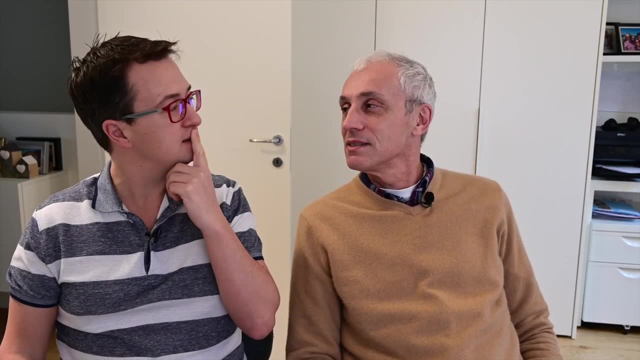 and that one requires a little bit of a transfer by taxi or by subway. but the rest of barcelona, i think we walked there and then taxied back. no, we took a taxi there and subway back. we did it. yeah, it was not, it was long, it's a long, long way. yeah, the only evil part of barcelona, it's quite. 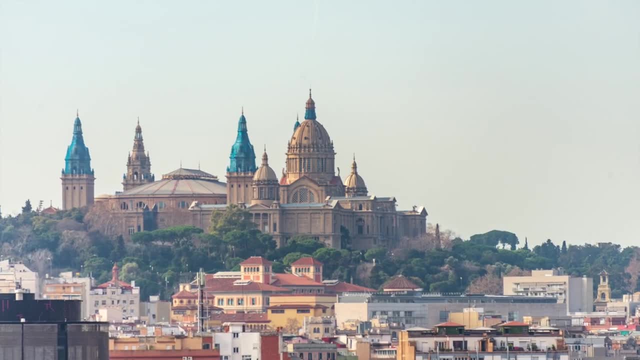 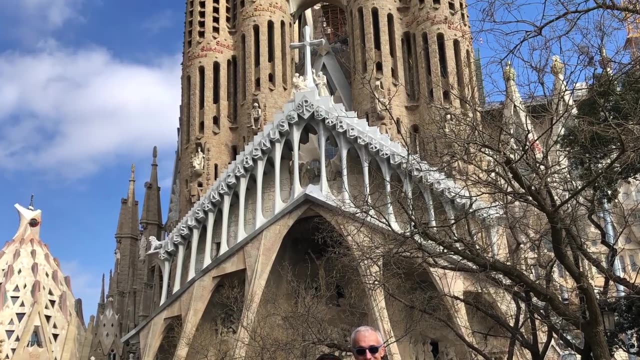 beautiful. i love it there. it's like so much fun and everyone wants to go see, obviously, the sagra, the familia. yeah, exactly, that's a bit of a stretch to walk there, but it's fun, i think. so i think i think that ought to be the first place that people ought to walk to at least younger 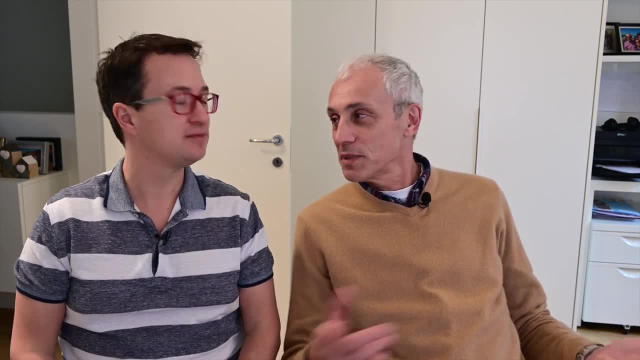 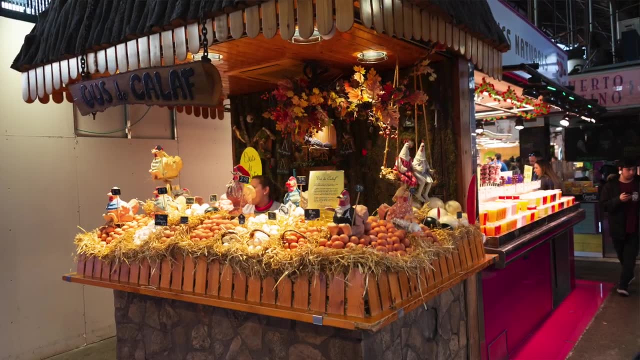 people, and then it builds up an appetite. that's a long one, and then you can stop at the market for lunch. exactly, yeah, the market on la rambla, oh yeah, it's beautiful, definitely, but go early, yeah, and you get really busy, definitely. another beautiful part: actually, the port itself is not 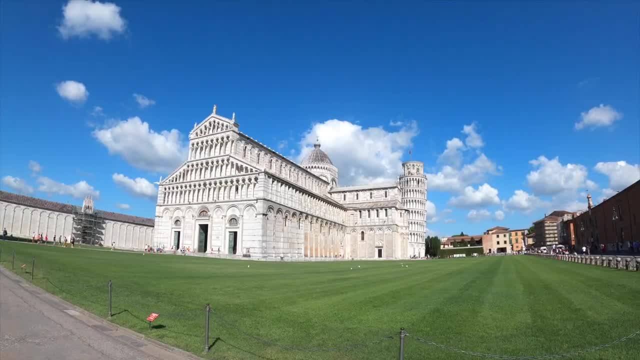 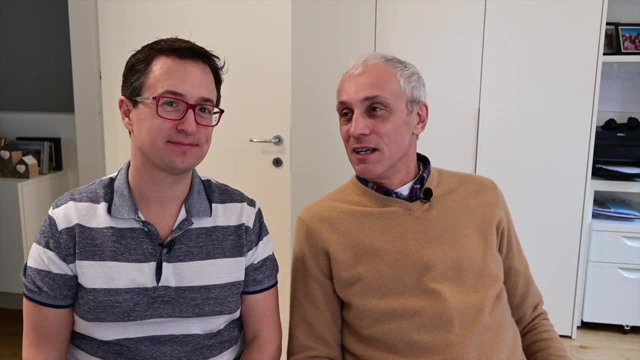 very beautiful. it's livorno, no, but it's the gateway to pisa and florence. yeah, no, there's nothing to see in livorno, but pisa and florence are very short, uh short, distance from livorno. you can take a transfer from the port to. 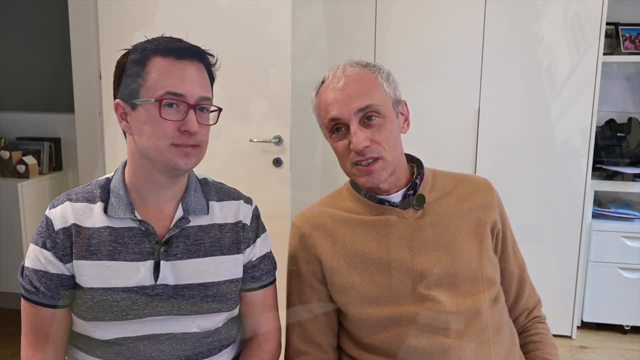 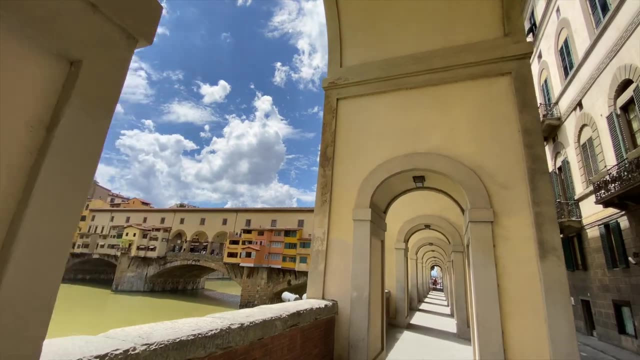 pisa- it takes about 20 minutes to get there. or florence: you have to take a train or a transfer. the key is: one or the other. yeah, one or the other, because oftentimes the cruise lines will have a tour for both in one day and 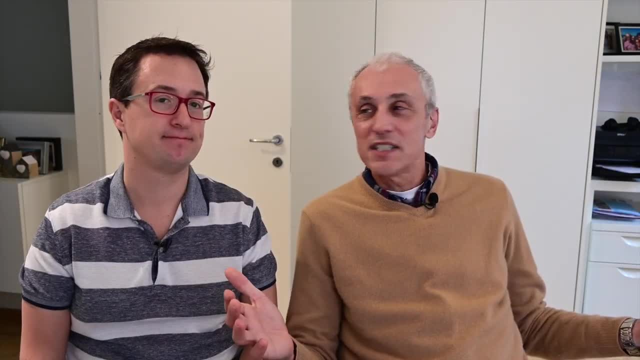 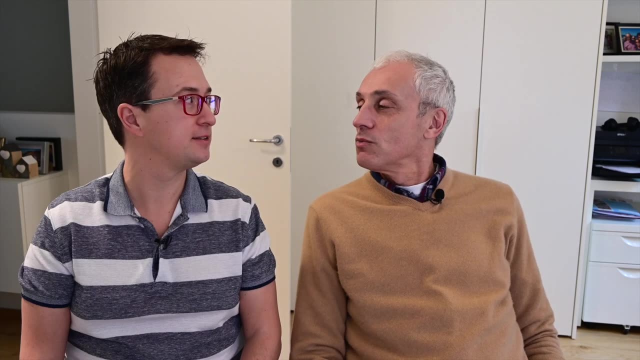 there's just no time to see anything. no, like florence itself can take like days to visit the whole like, so you won't see anything. really, just take your time. good advice, which one's your favorite? well, i like. yeah, i like geneva as well. i mean, i remember geneva having the, the focaccia. 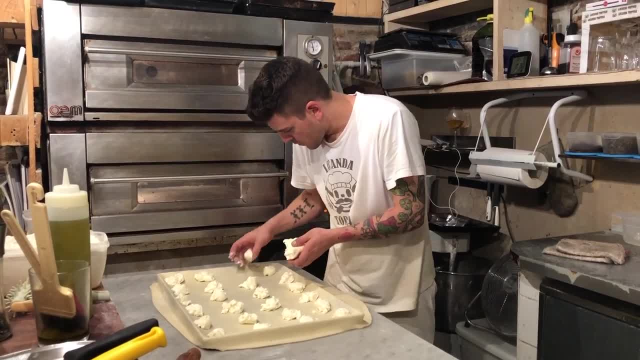 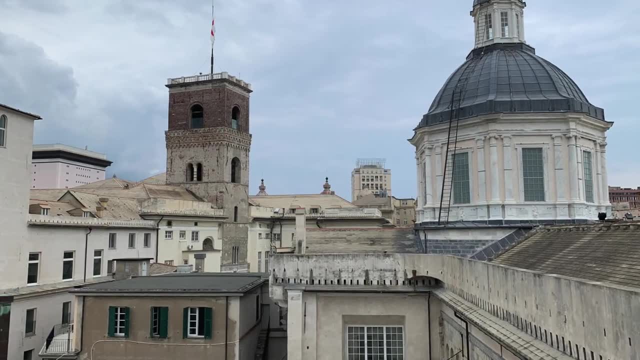 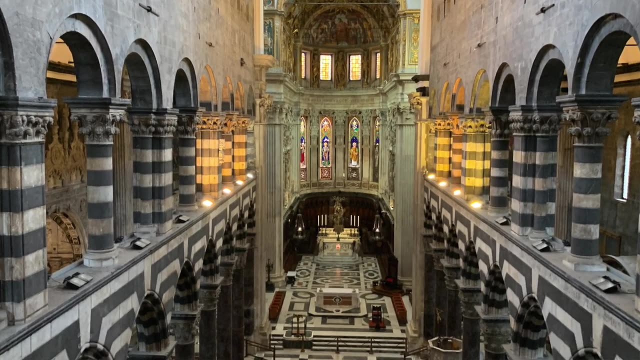 oh yeah. yeah, that was, that was an interesting. that was an interesting stop. even though we live in italy, uh, geneva is just not a city that we we tend to visit, but it reminds me a little bit. actually. it's quite nice with the duomo, and there's lots of cute restaurants that you can actually stop for. 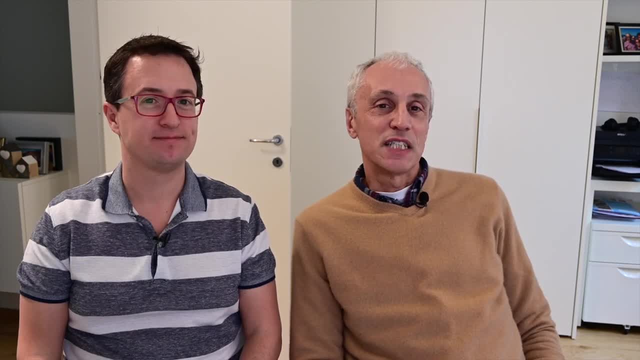 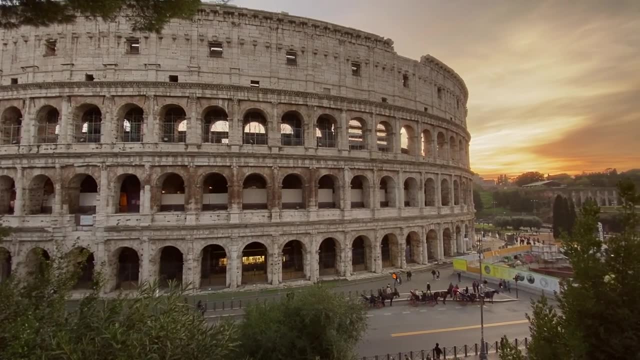 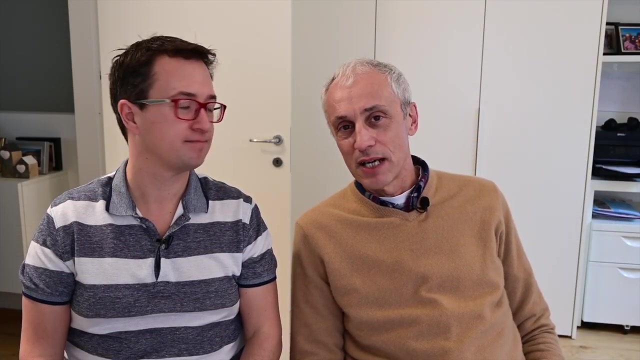 lunch, sure quite fun, definitely. and then there's chivitavecchia, which is the gateway to rome. right, don't go to the mcdonald's, just take a trip to rome and enjoy it. yeah, it's about an hour outside rome. you can take the train there, take the road, the train to the downtown rome. it's like. 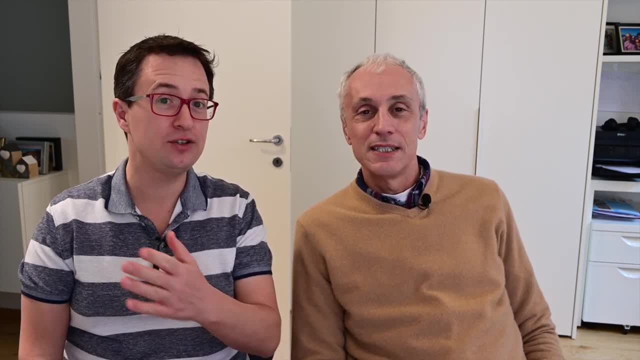 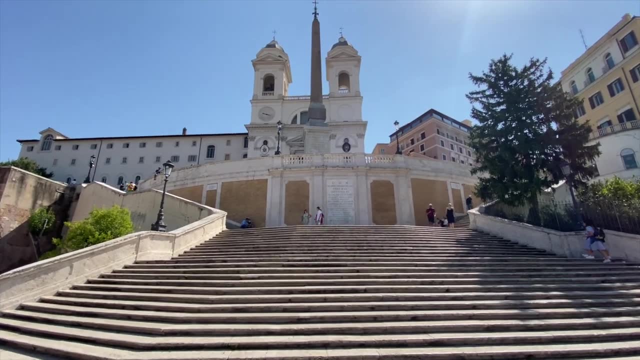 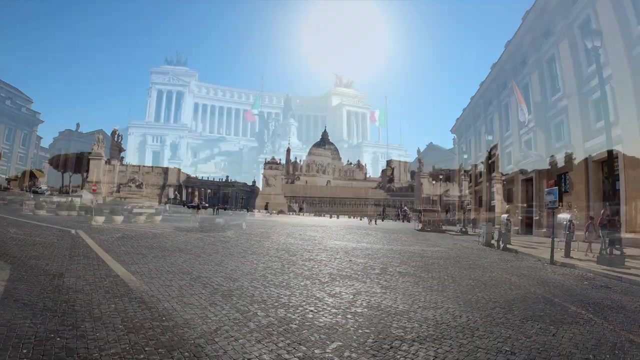 right train, right like really convenient exactly now. if you have never been to rome before and you find yourself at the port of chivitavecchia wondering what you should do, well, i highly recommend that you do a little bit of research. yeah, because if you just arrive and you take a transfer willy-nilly into 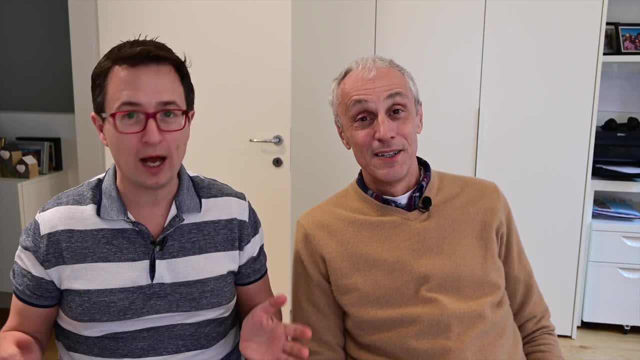 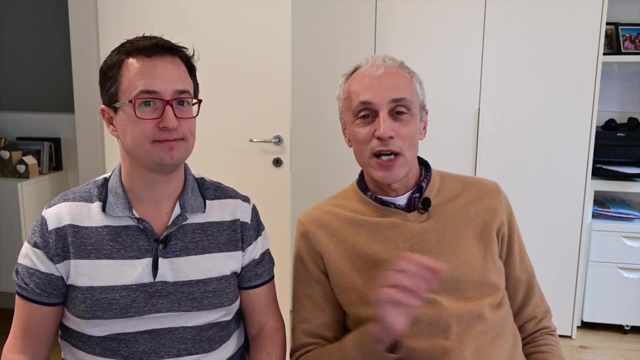 rome, you're going to be like, you're going to be overwhelmed. you'll have no idea what you're looking at. very well, run in the city. so and again, again in rome, be focused. don't go, don't try to go everywhere. just pick three or four main landmarks and visit those exactly. 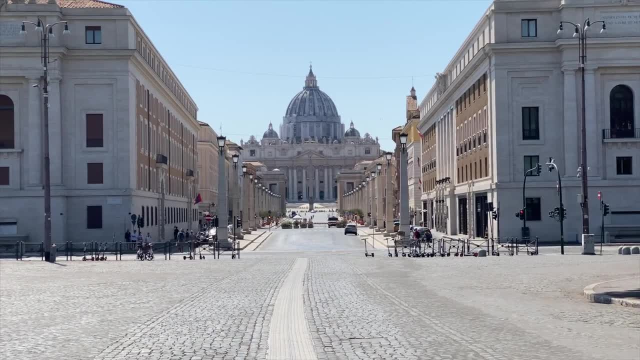 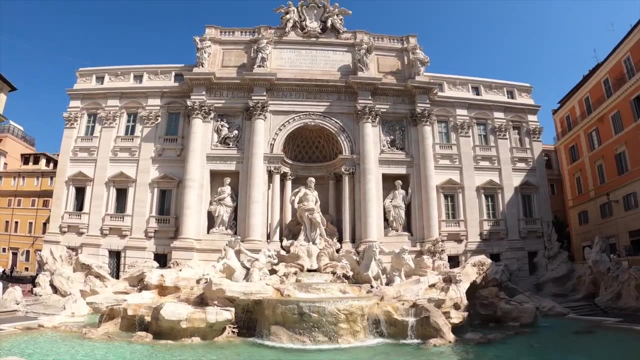 you can go to the port of chivitavecchia. so if you are going to rome, it's possible to see everything in monday, yeah, definitely, but you can see, you know, probably the colosseum, the trevi fountain and the pantheon, the pantheon, and probably you can go, you know, maybe, uh, to the vatican. 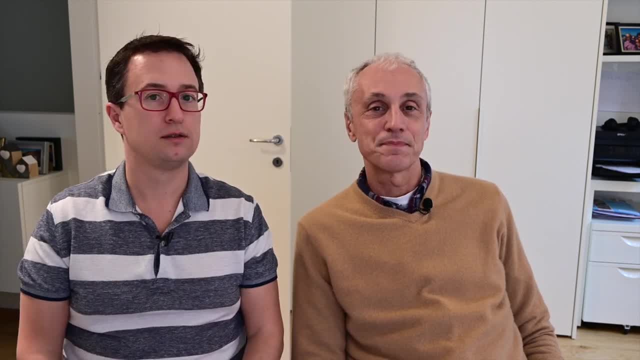 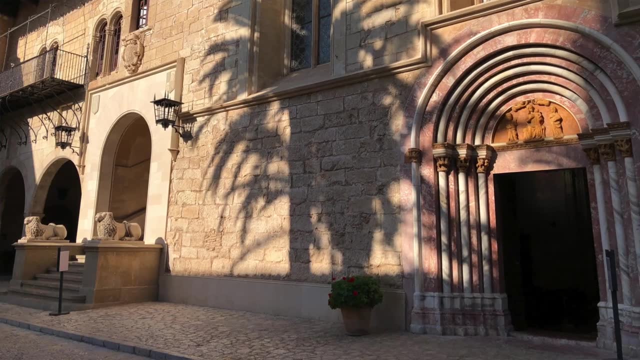 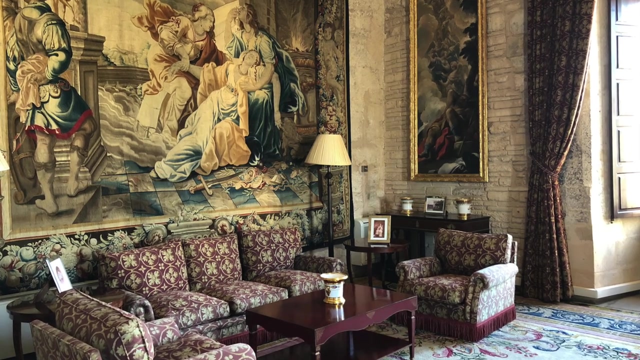 not, not the vatican museum, no, no, no, that takes a day. no, you can go to the square, yeah, so yeah, and i like palma de mallorca. there was another fun port. yeah, we got to visit the uh president palace. yeah, The Duomo is beautiful. It's such a huge little island and it was beautiful. It was February and mid-20th. 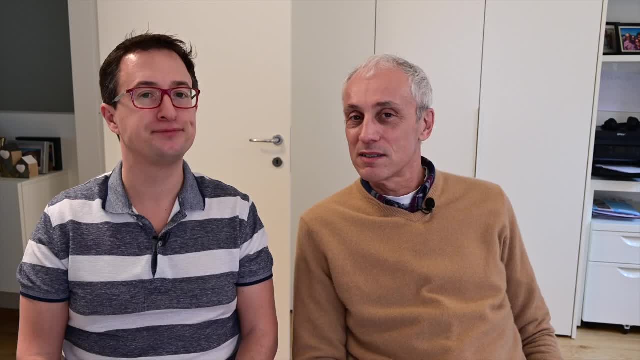 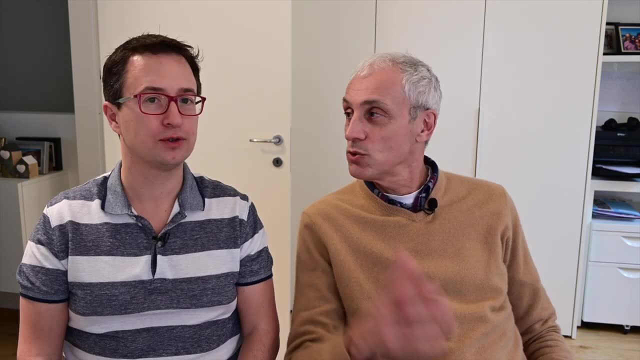 Yeah, we did that on a Costa cruise. I know I loved that stuff. I really, really enjoyed it. These were some of our favorite Western- Yeah, Western- Lithuania ports. Let's go to the Eastern Lithuania, All right. Well then we have Venice. Who doesn't like Venice? 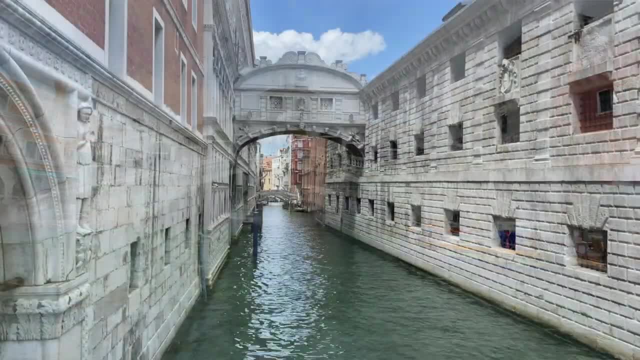 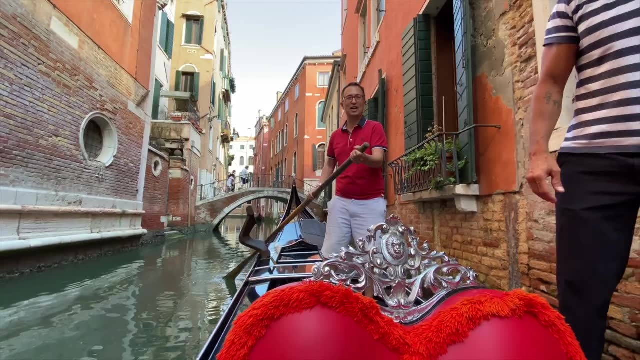 Yeah, who doesn't love Venice? Venice is a spectacular place And you know, if you come to Venice, one of the things that you might try doing is row the gondola, Row the gondola. yeah, With a little smoothing of the gondola here. 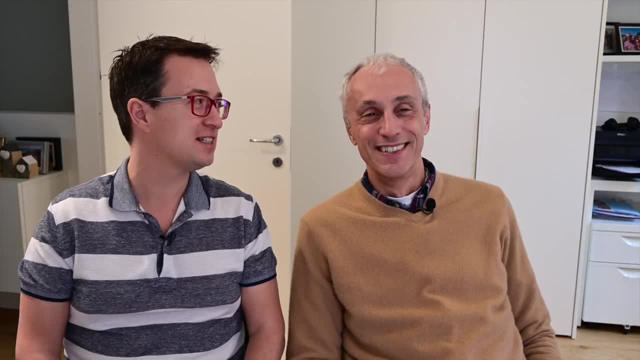 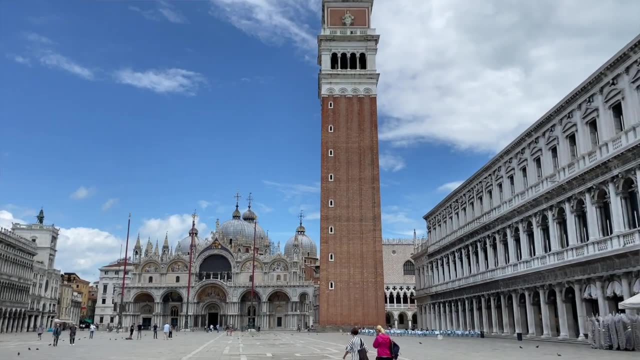 Yeah, you might need, like a, A grumpy- I was going to say a Benjamin, but sure you could try. Exactly, Venice is definitely beautiful. Again, try to explore the city and don't try to do everything in one day. It's impossible. 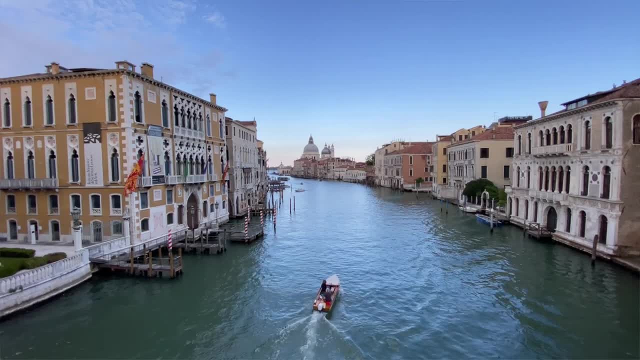 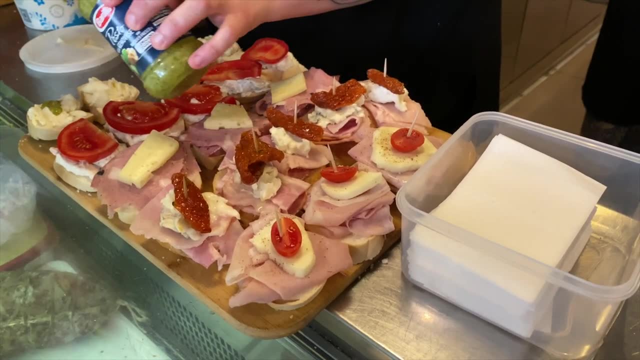 Exactly So. pick a few little places, Pick a few spots, and go there And go and eat those cicchetti Oh, cicchetti, Yeah, Those are beautiful, Absolutely. Unfortunately, there are rumors that Venice is not going to be a cruise port anymore. 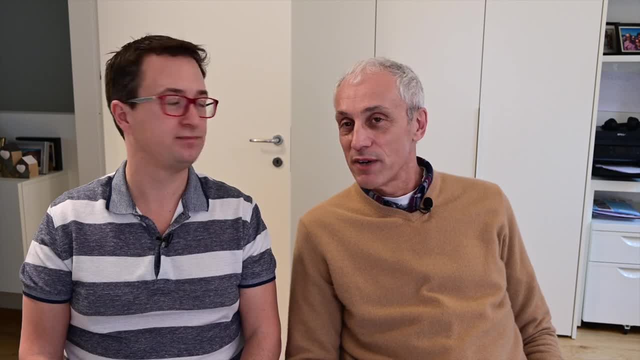 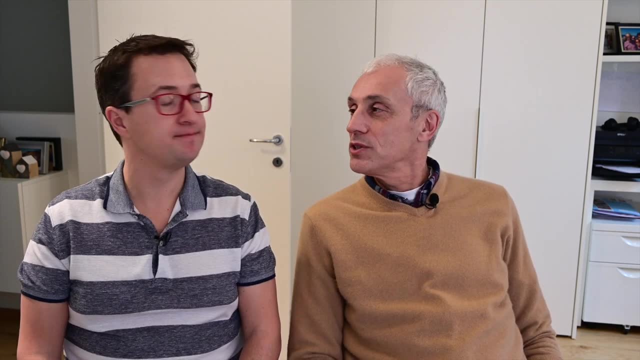 They might move the cruise ship outside Venice because of the environmental issues, So there might not be a port in the Med anymore. We'll see, Yeah well, we'll see Another port on the Eastern Mediterranean: Athens. Athens is, It's like the Rome of Greece, right? 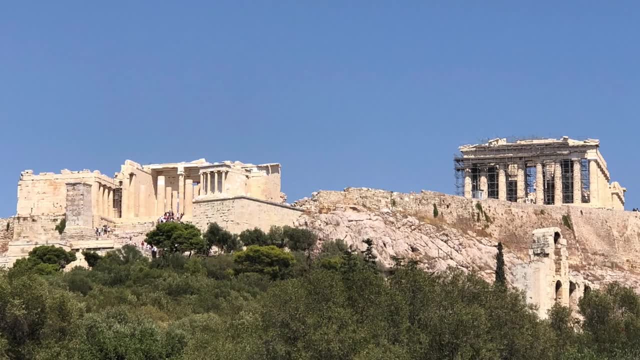 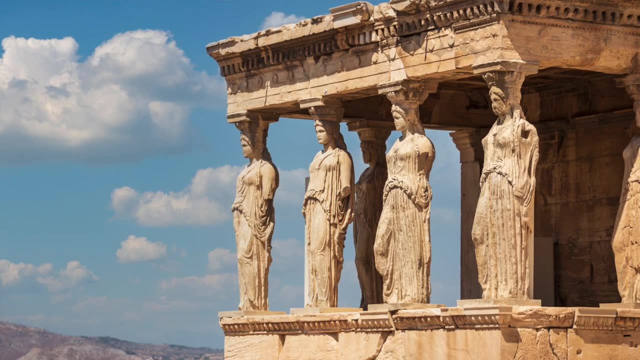 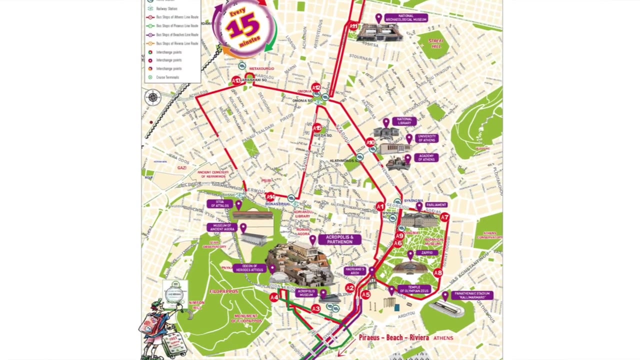 Yeah, I mean, it's like It's just another one of those cities that you need to go there with a plan or with a guide. Actually, I deeply enjoyed the Hop-on Hop-off bus. That was perfect. actually, The Hop-on Hop-off bus is usually a fan favorite because you get to see a lot of nice things and then you can stop. 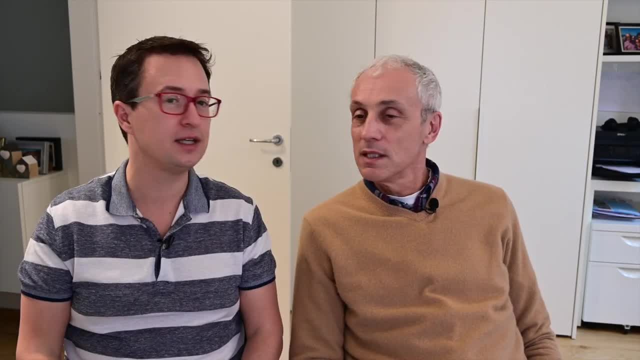 And they also have a guided. They have a guide. You put your phone- Your phone, yeah, Exactly. You can listen to what You know, what The guide talk about, what they're, What you're seeing, And you can catch it right in the port. 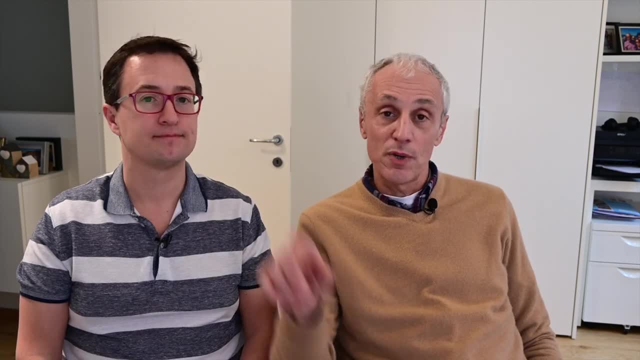 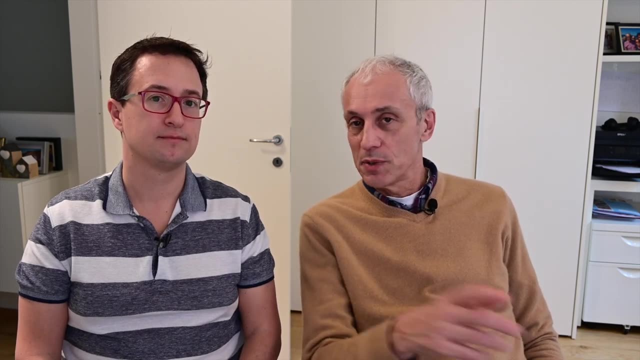 So it's very convenient. You catch the Hop-on, Hop-off right in the port, which is about half an hour outside downtown, And it takes you downtown and shows all the stops and you can stop in one place and get on in another place. 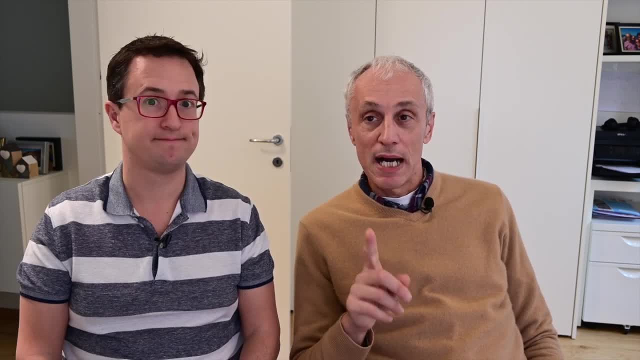 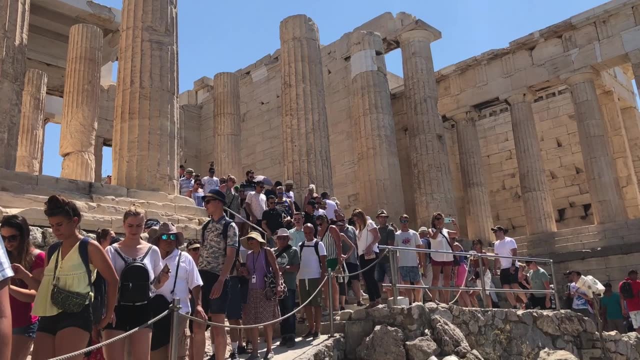 It's perfect, actually, Right, One thing that you have to do in Athens: Buy the ticket for the pass and on in advance. Yeah, I haven't been lying. Yeah, It just goes on and on. It's just like ridiculous. 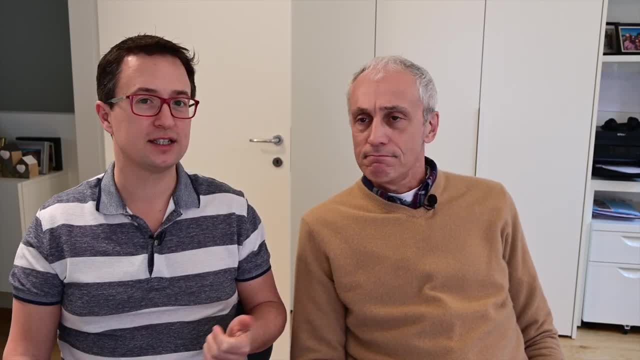 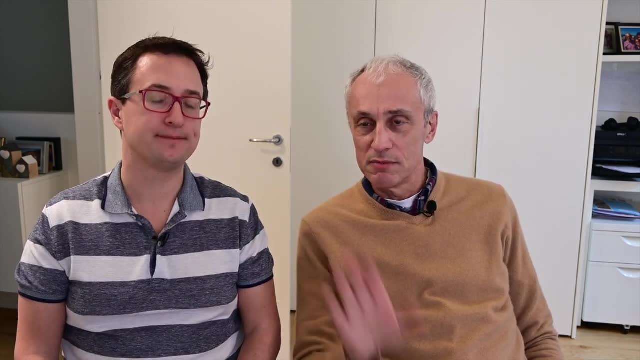 Unless the cruise sells it. But if the cruise sells it it's going to be far more expensive. I went on the website and it took me like five minutes and we arrived at the pass and on and we got our barcode and went in. 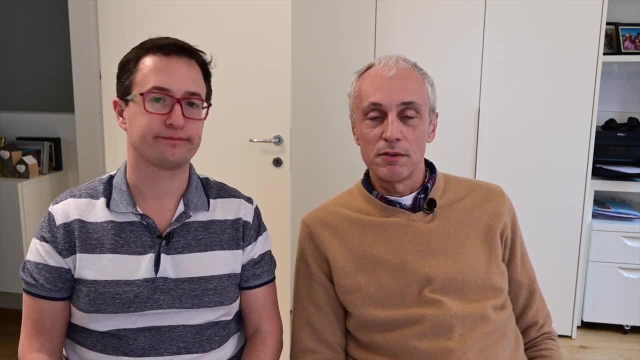 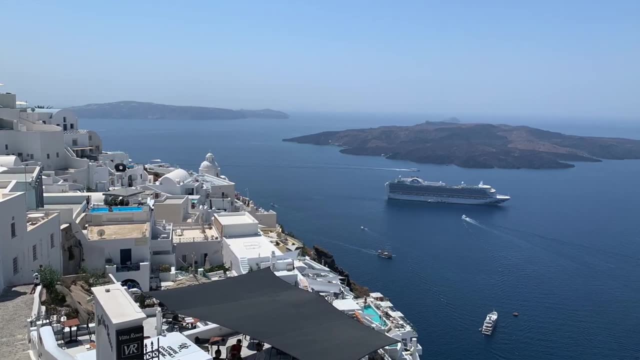 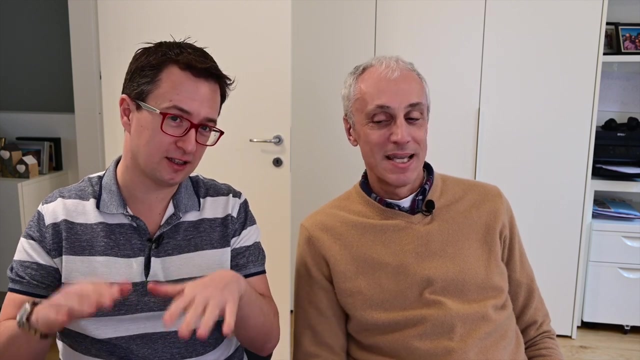 No problem, Yeah, And we did that. one on our own. Yeah, Yeah, Both on our own. And then, who doesn't like Santorini? Santorini is spectacular, So beautiful, Spectacular, So so beautiful. Take the gondola if you don't like donkeys or if your mobility is a little wonky. 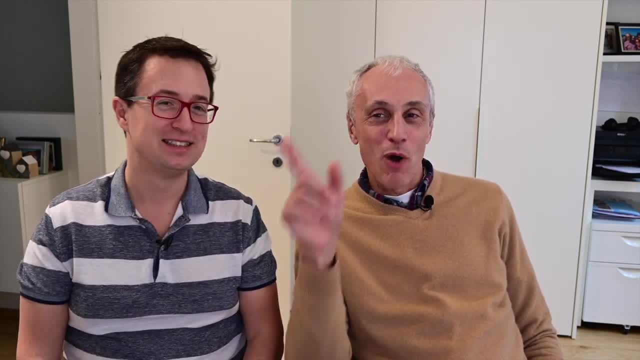 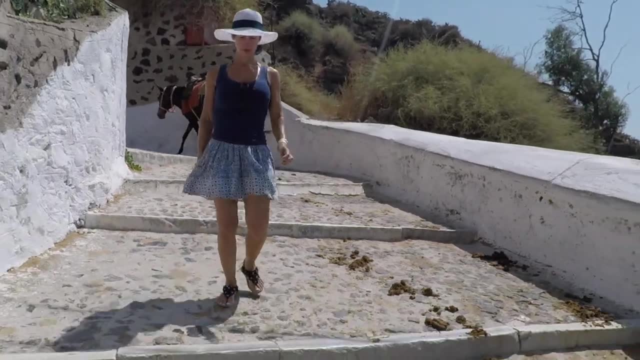 Yeah, Yeah, We were walking down the cliff. Yeah, We were talking about what the donkeys are and what slightly slippery do the donkey droppings, Donkey droppings. This one slipped in the donkey droppings. 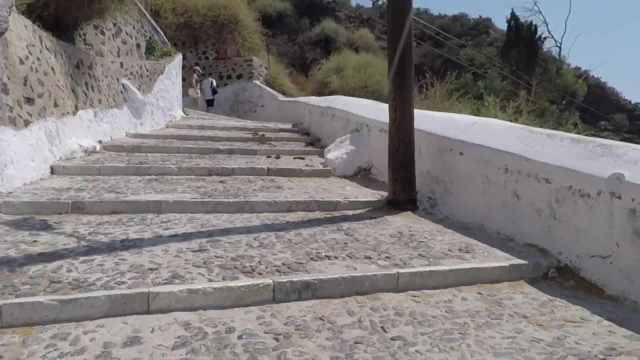 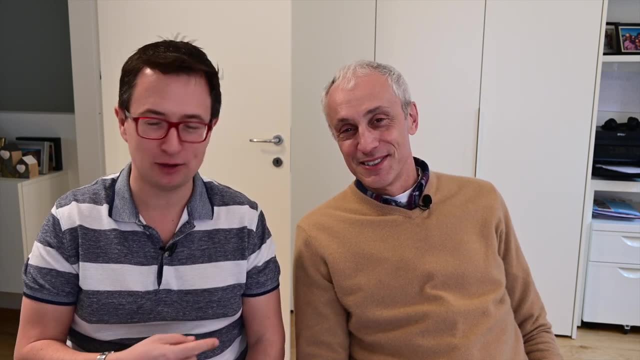 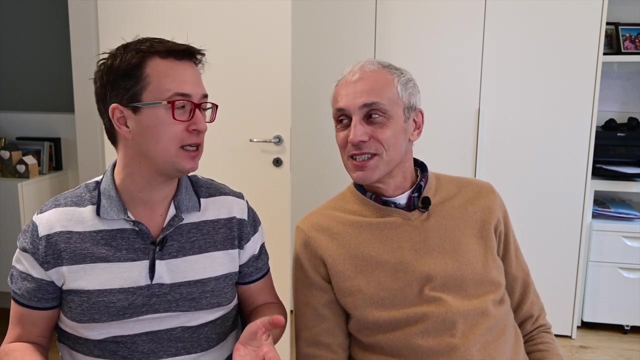 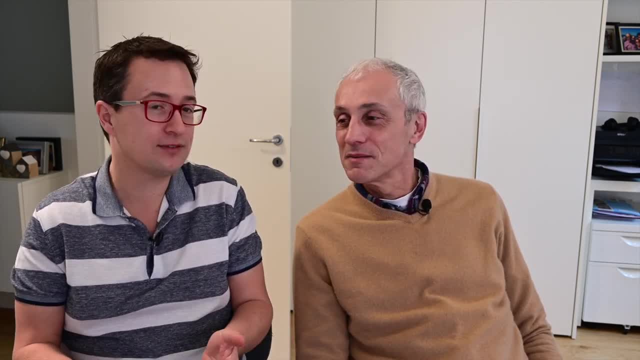 Look, the last time I was there was in 2007 or something like that, And it was a lot different in my memory. But Yeah, No, Yeah, Probably because you asleep in a donkey droppin, that was probably different. 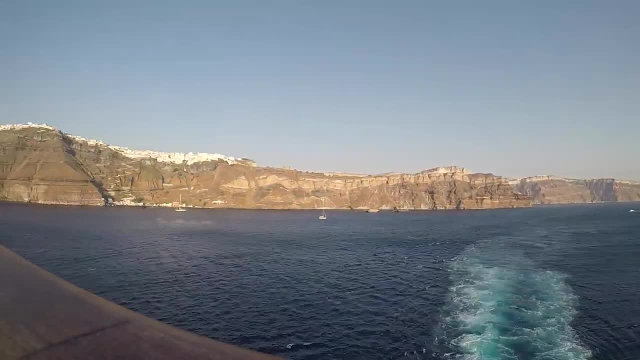 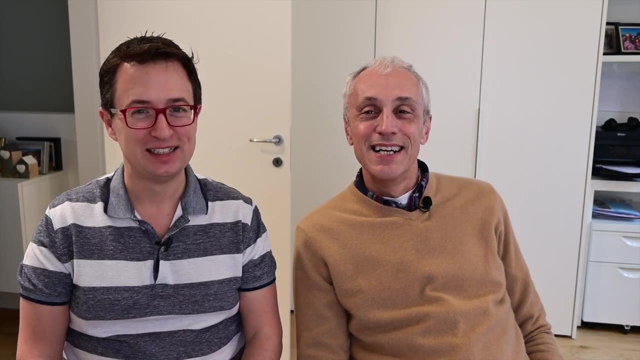 Probably No, It was a lot less slippery, definitely, Definitely. So yeah, Well, maybe I might ride the donkey More. Yeah, Yeah, Maybe I'll take the gondola. And how about Mykonos? 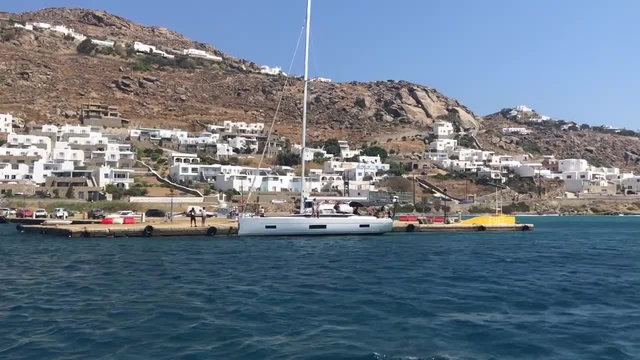 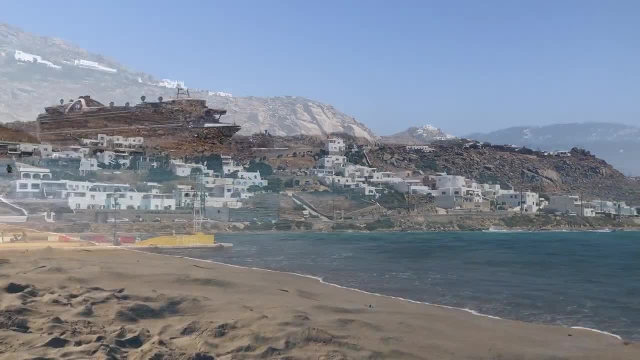 Oh, Mykonos. Oh Now, Mykonos is freaking expensive, Really expensive, but it's really cheap. But if you go, if you dock at the new port in Mykonos, there's a beach right there just. 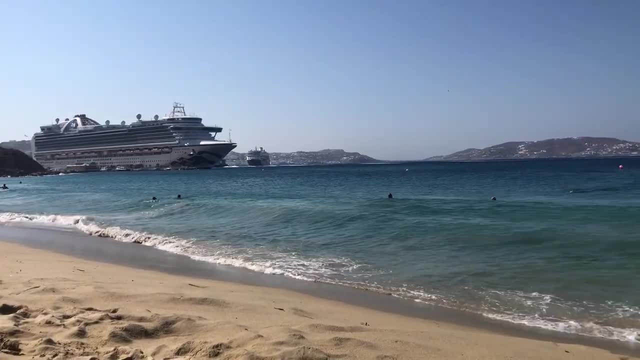 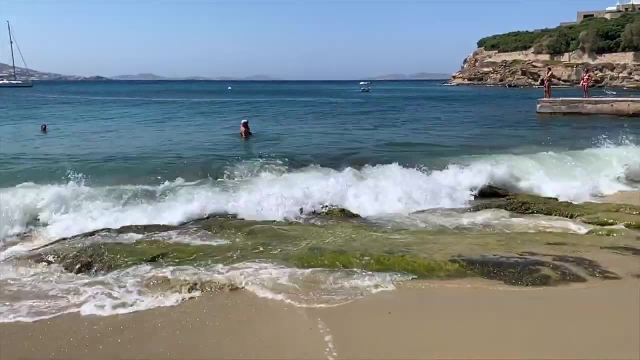 crew members that know this. It's like a five minute walk. It's called St Stefano Beach. Yes, you don't have to take any transportation, just walk there, just up the hill, down the hill. Yeah, and it costs almost nothing. 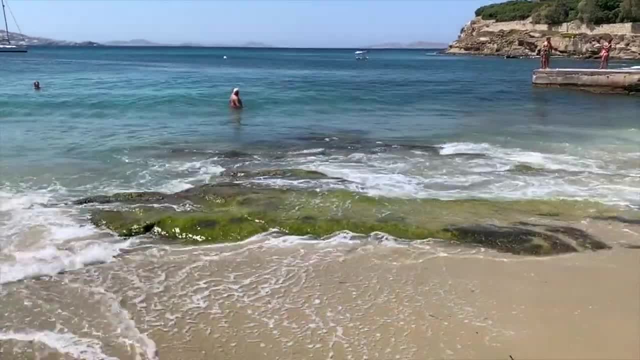 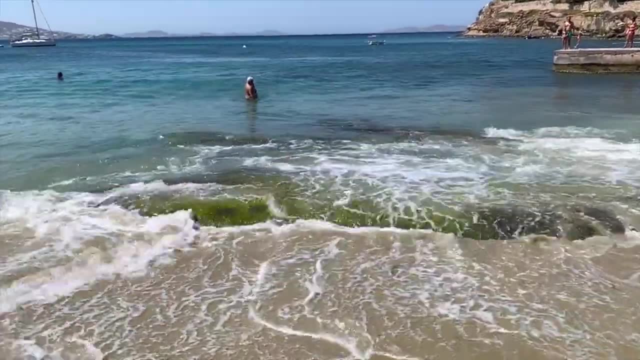 I think we paid like 20 euros for the entire day. Oh, beautiful, And there's restaurants there. you can sit there, have a nice Greek meal. it's absolutely fantastic. The water's fantastic. The water's fantastic And warm. 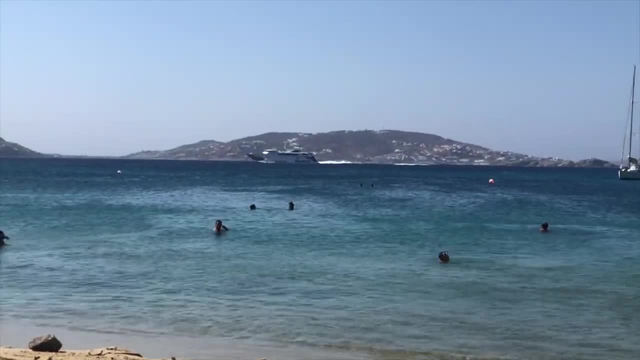 What do you mean? Well, yeah, it's because they have these fast ferries that go by close by and they make these gigantic waves, But actually it's fun. Yeah, it's fun, It's actually quite interesting. 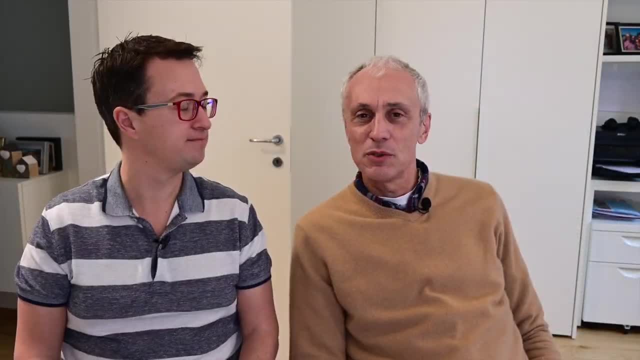 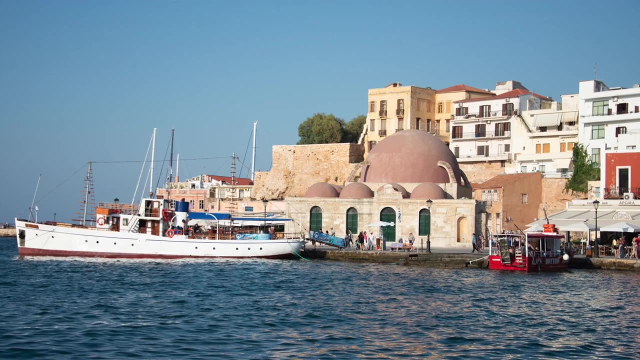 Oh, I love the beach. It was really beautiful, Definitely. And then we went to Crete. I really loved Crete. It was beautiful there too. They were very honest people there, Very nice, Very honest people. You remember when I lost my cell phone? 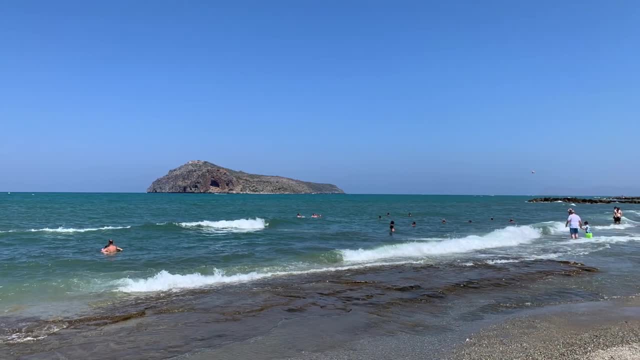 Yeah, I remember. Yeah, I know They brought it back to the ship. I know, Incredible, It was really really nice. Yeah, No, we loved both southern and Mediterranean. We did enjoy them both And we can't wait to go back. 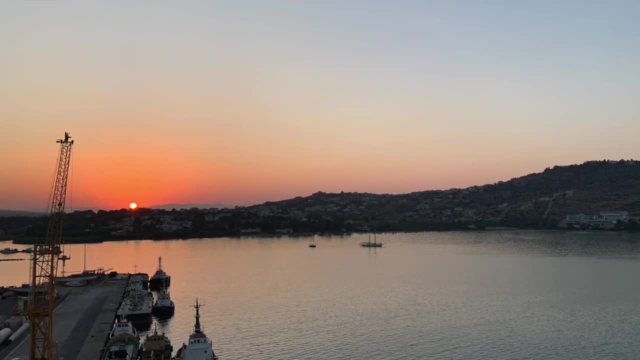 Go back. Can't wait to go back. I mean, we're on standby, Yeah, As soon as we're able, we're, We're going to be gone and you're going to see a video of us in our ship. 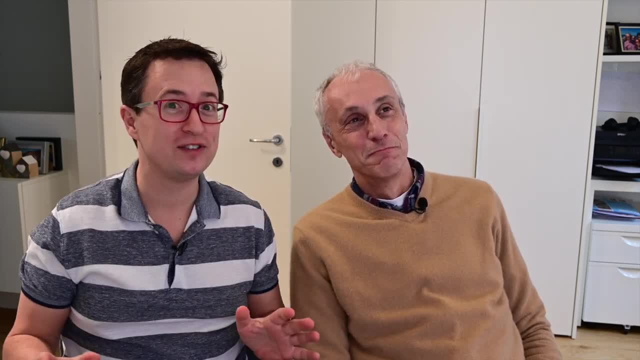 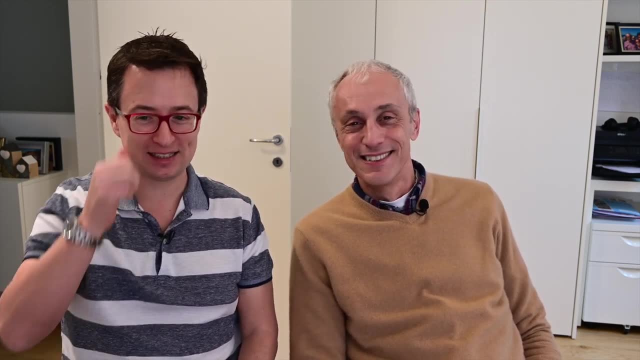 Exactly, And it won't be old videos, It'll be new videos, It'll be Exactly. You'll probably see this B-roll footage like a few times: Exactly, Exactly. Well, guys, which one was your favorite out of all of these? 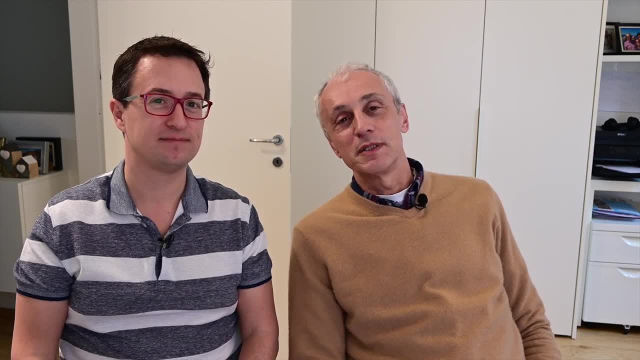 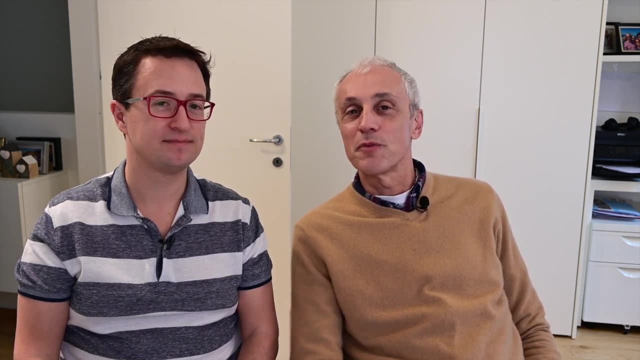 Exactly, And if you want a complete list of all the ports on the Mediterranean, follow the link in the description. There's going to be a super expensive list of every single port in the Med that you can visit, with lots of description. That's great advice. Now you might be wondering: should I do a one, two or three-week cruise? Or how long should you be on a Med cruise? Yeah, three. In our opinion, the longer the better, especially if you're coming all the way from North America. 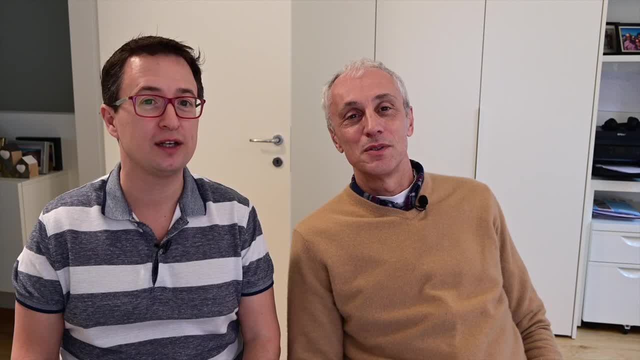 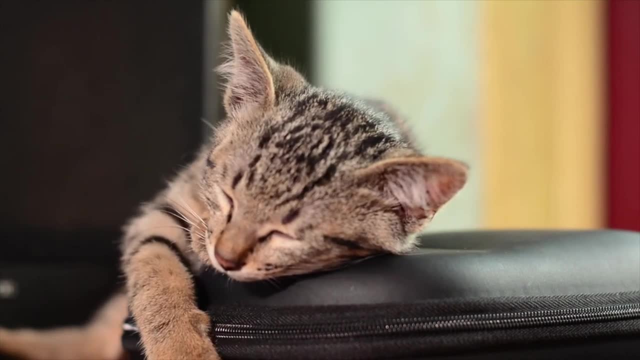 The minimum you should plan is a two-week cruise, Because the first couple of days you're going to be dealing with jet lag. Yep, And, by the way, if you want to know our tips with dealing with jet lag, check out the video. 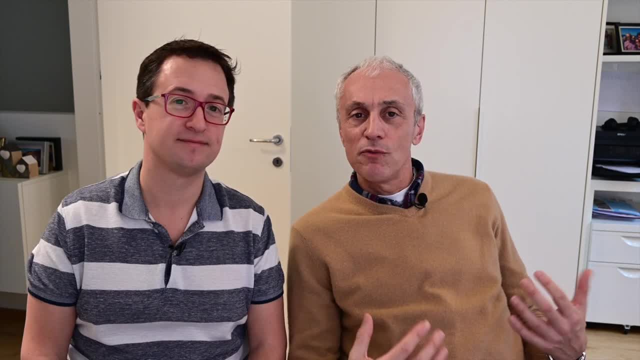 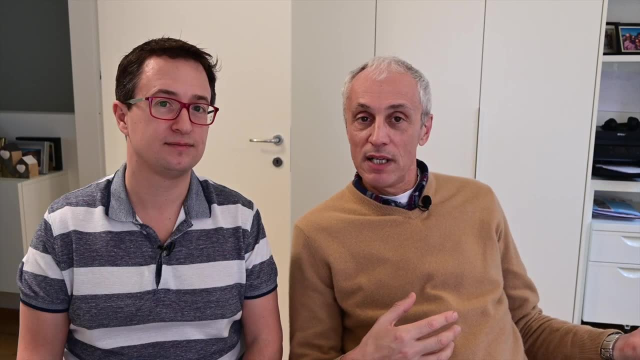 Yeah, one-week cruise are usually cheaper, but they don't visit as many ports Like two three-week cruises. they visit way more ports. So we tried both seven days and we tried 21. And we loved them both, but 21 was absolutely fantastic. 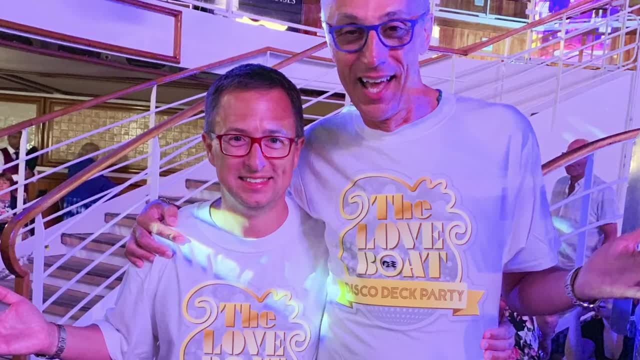 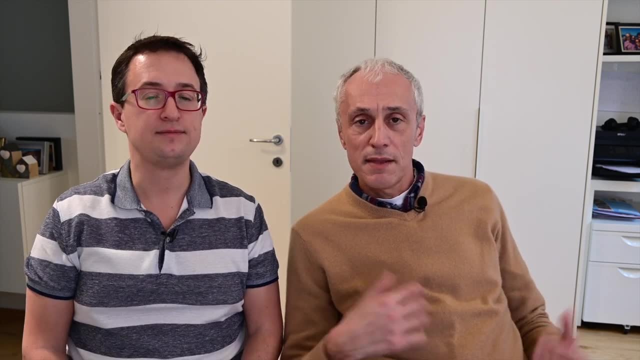 And you remember, you become part of the crew. Absolutely So, in our opinion, the longer the better. So book, the longer you can afford and you will really like it, Mm-hmm. Another thing you want to consider is if you should take a one-way cruise or a return cruise. 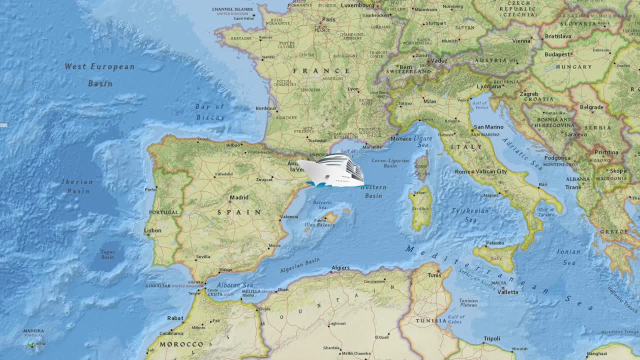 The difference is very simple. In a one-way cruise, you go from one port to another, So you embark in Barcelona and disembark in Ciutadella, While on a return cruise, the embarkation port and disembarkation port are the same. 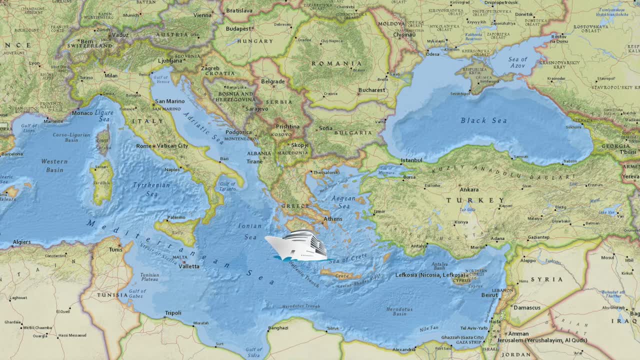 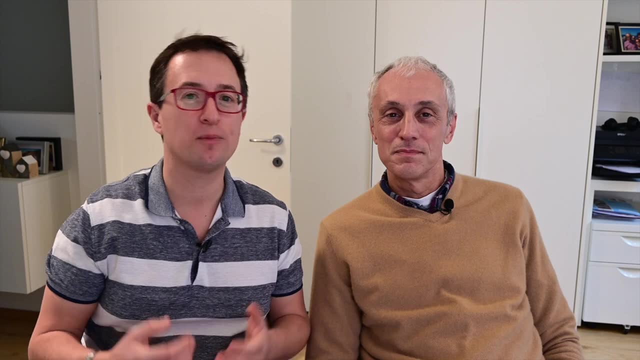 So Venice to Venice, for example, Athens to Venice, Athens to Athens- Advantage on the advantages. The advantages of a one-way cruise is the fact that you'll be able to visit more ports, as these type of cruises are usually longer than seven days. 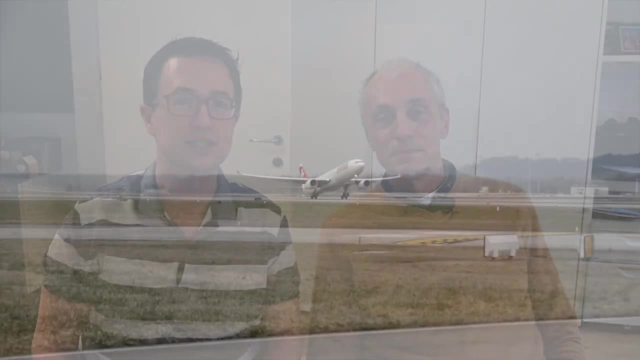 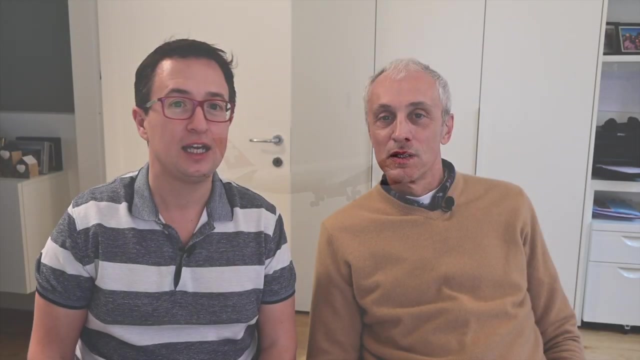 The biggest disadvantage of a one-way cruise is the fact that the flight might be slightly more expensive, since you arrive at one airport and you leave from a different one. If you choose a return cruise, these types are generally one week long and they circle around six or seven days. 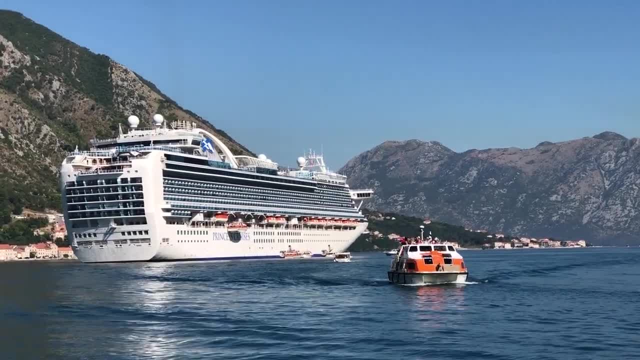 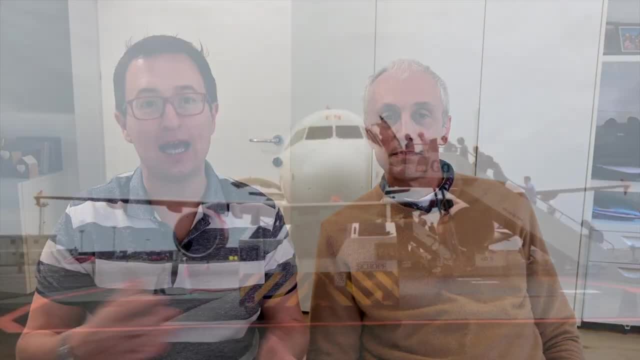 They circle around six or seven ports in the same area, For example, they're more popular in the Greek islands or the Adriatic, And they have the advantage that you're flying in and out of the same airport, making it easier to find a cheaper flight. They're also cheaper most of the time because they're a shorter cruise, So that's a big advantage. Last thing to consider is what is the best season to cruise the Mediterranean. Most mainstream cruise lines around the Mediterranean are between April and November, And if you're looking to enjoy the sun, swim in the Mediterranean or go to the beach. the best time is the middle of the summer, June to September, when the water is warm and the weather is warm and the sea is usually calmer because there's no chance of storming that season. Unfortunately, this time of the year is also the most expensive and the most crowded. It's also the hottest time of the year. It can get to over four degrees, It can get to over 40 degrees Celsius, making visiting cities a little bit uncomfortable. So if you're looking for visiting cities and doing more sightseeing, the shoulder season is a better option for you. In fact, early spring and the fall are cheaper, They're less crowded, The temperatures are better, But on the downside, the weather might be more unpredictable and chances of rain are higher and the sea can be rough. And there are two main cruise lines. Costa and MSC, which are European-based, do the mad rear round even in the winter. The Mediterranean cruise in the winter is a completely different experience. It's still very enjoyable, In particular if you take a cruise that goes way south, like to the Greek island, for example.